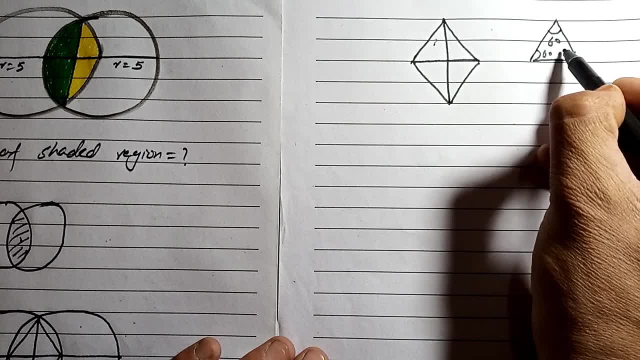 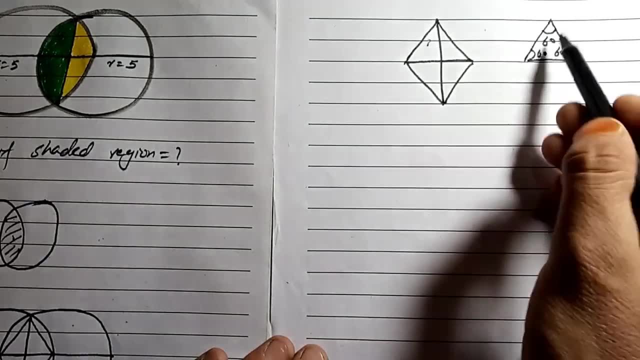 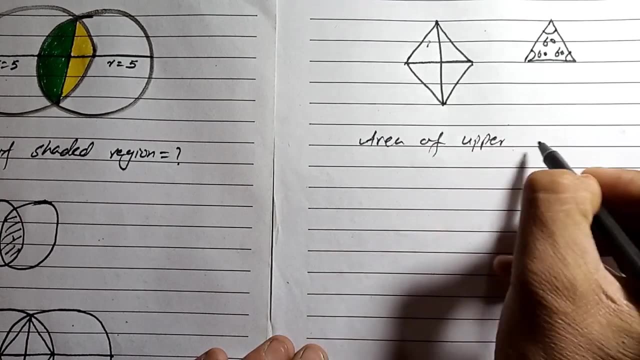 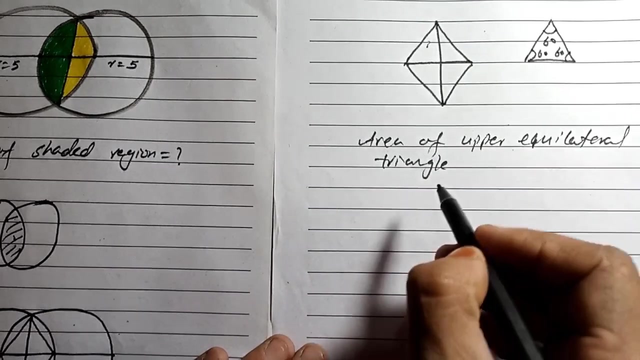 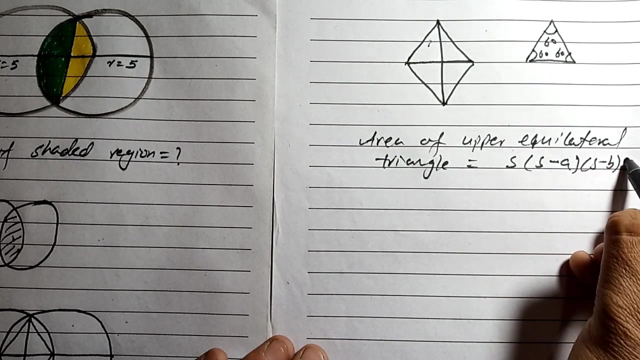 so this is 60, this is 60 and this is 60 degree, so we can find the area of upper liquid equilateral triangle. this is so area of upper equilateral triangle, so which is equal to s, s minus a, s minus b, s minus c. 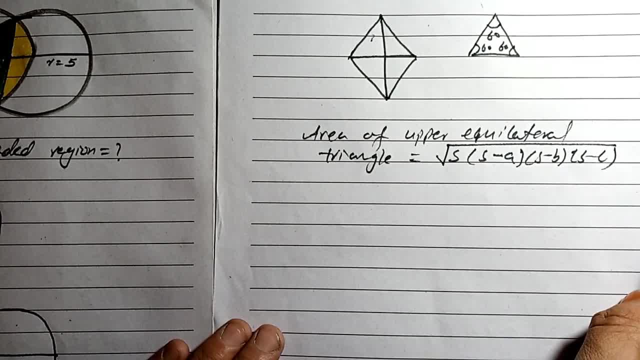 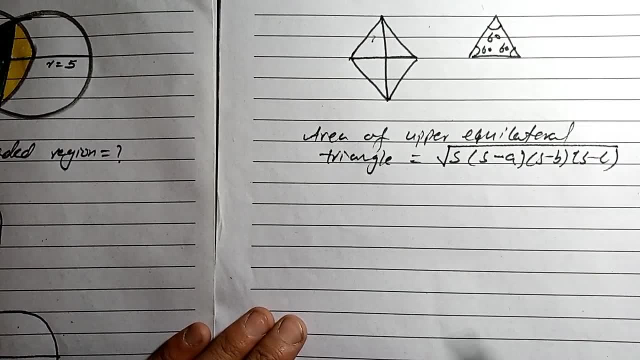 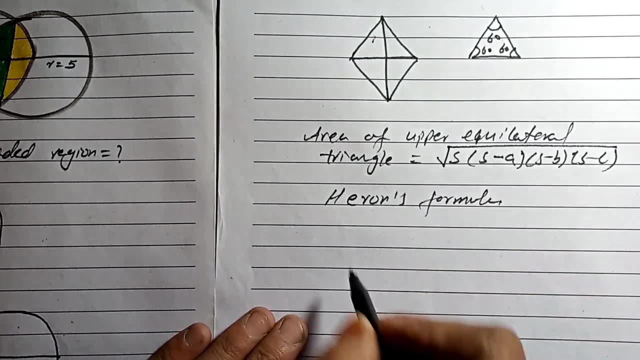 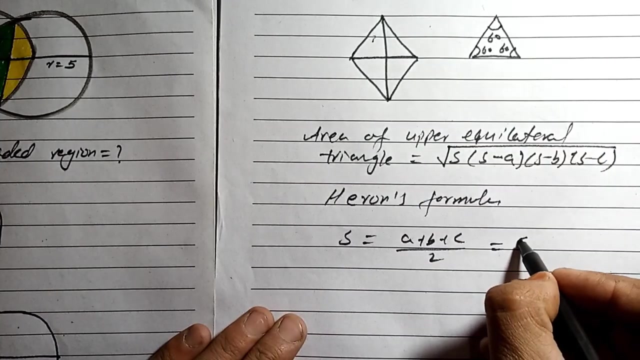 so equilateral triangle, having each side have same side length, so each side length is five unit. because, given that five unit, so we are using here in formula, here in this formula, which is s, a plus b plus c divided by two, so a, b, c also same unit, so five plus five plus five divided by two, we can get which is equal to: 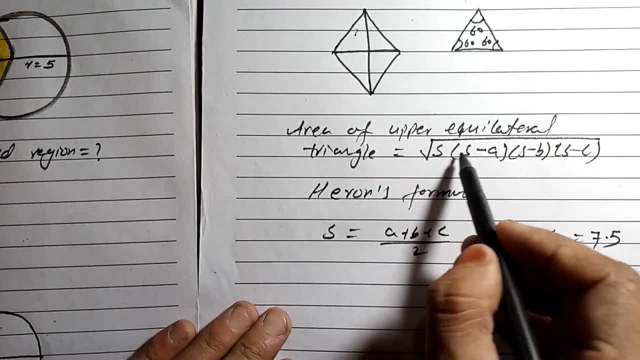 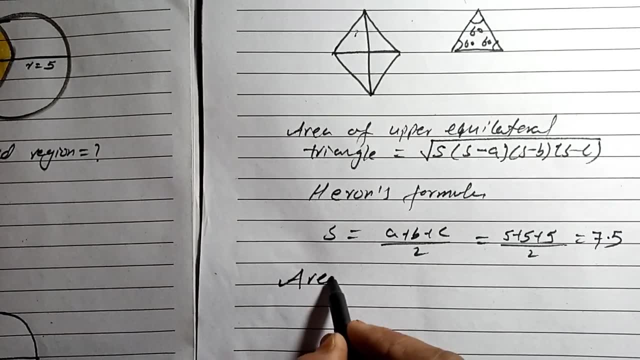 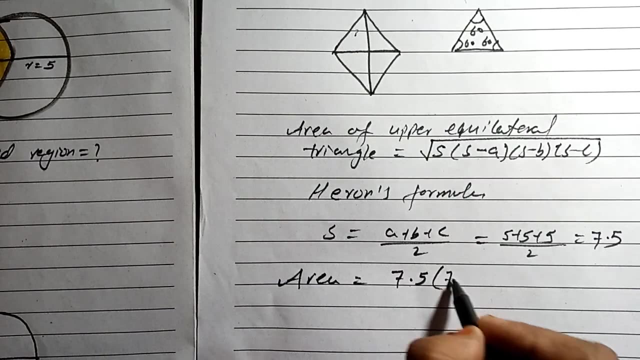 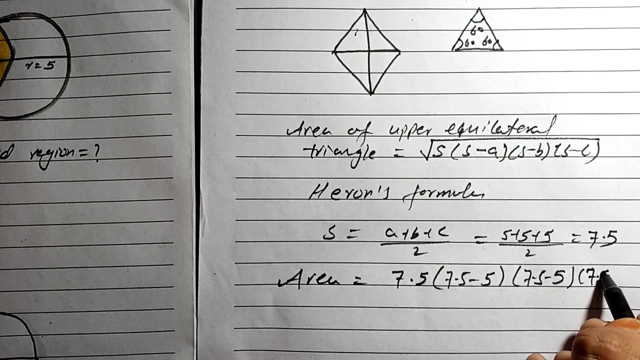 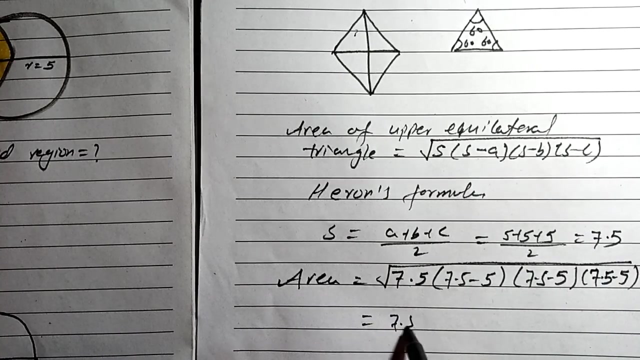 seven point five. so putting this we'll use, we can get the area of upper equilateral triangle. so area will be equal to s 7.5 and a s minus a, 7.5 minus 5, 7.5 minus 5, 7.5 minus 5 root, so we can get 7.5 multiplied 2.5. 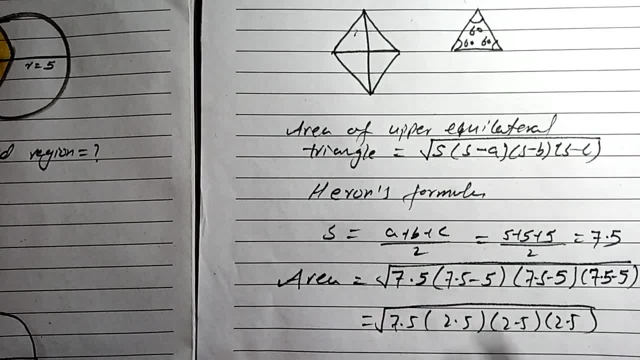 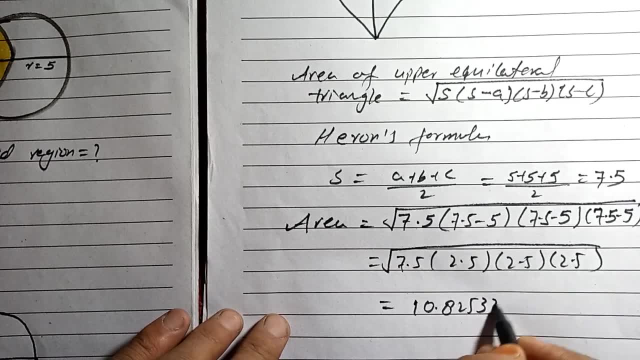 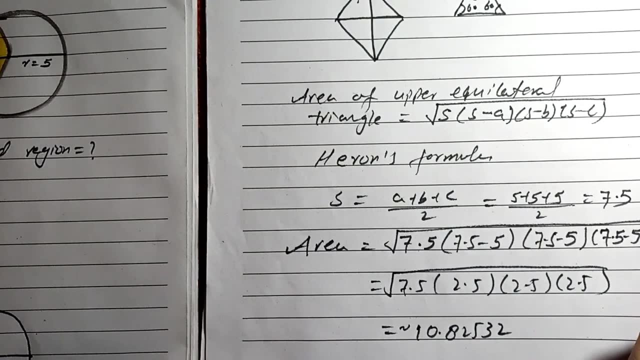 2.5, 2.5, so we can get approximate value, which is equal to 10.8283, to, which is approximate value of this area of upper equilateral triangle. so, uh, the total rhombus is equal to 8.2, which is: 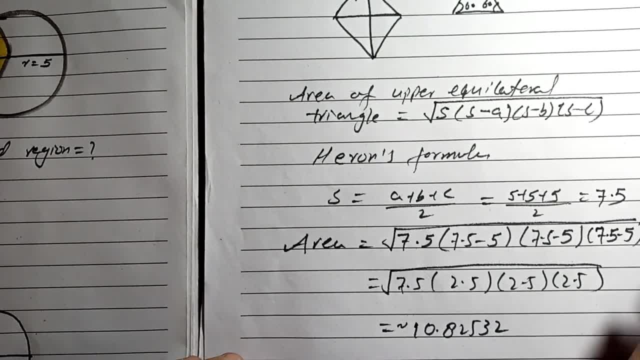 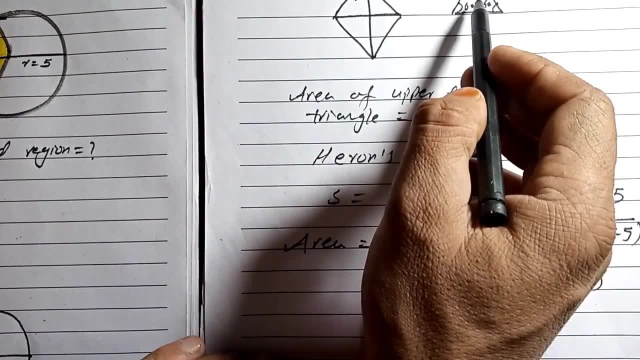 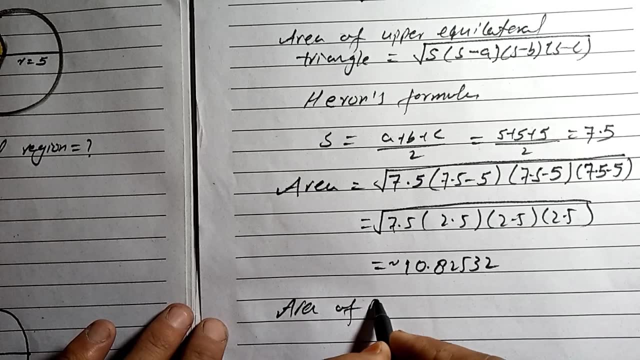 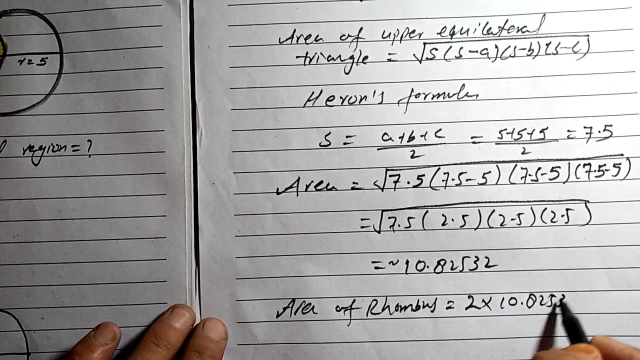 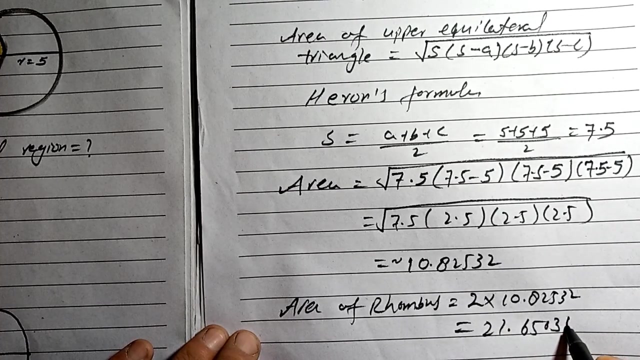 is equal, equal to two times of the equilateral triangle, this total area of this rhombus, which is two time of equilateral triangle. so the area of rhombus, area of rhombus which is equal to two times ten point eight, two, five, three, two, which is equal to twenty one point six, five zero, three, five zero six. 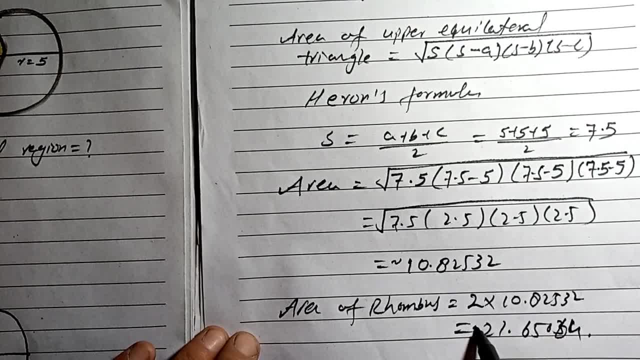 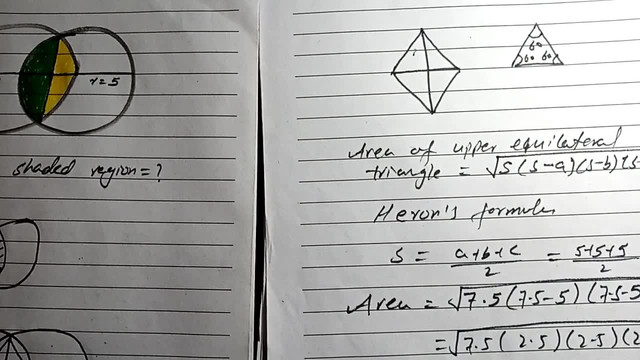 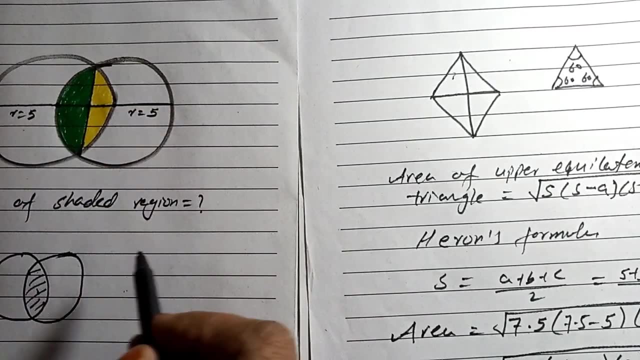 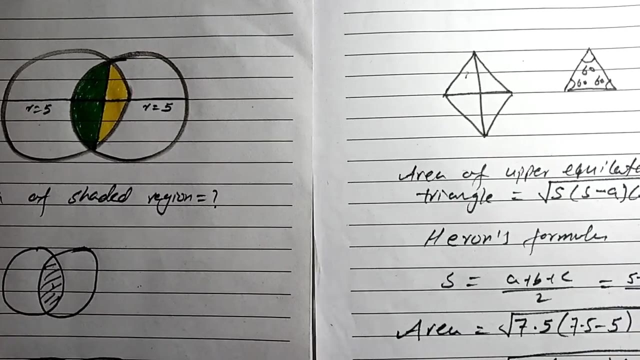 four, six, four, which is approximate area of this rhombus. so our main aim is to find the area of this shaded region. so we have left the. if we convert this into any this we can get the area of this region. and we have left this for a side. only left this for side, we can get the. 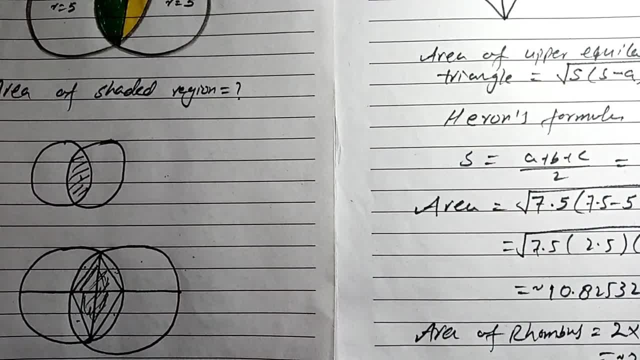 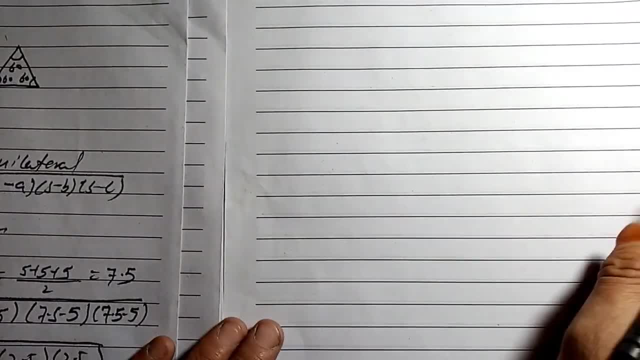 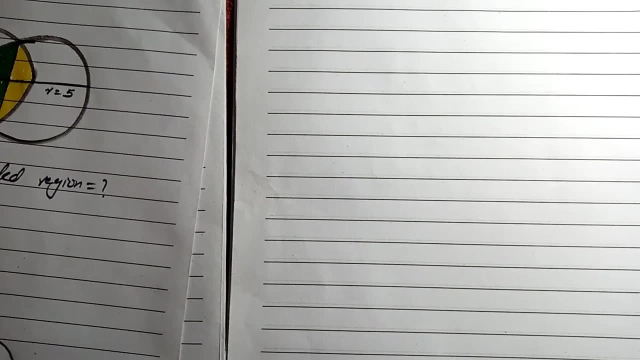 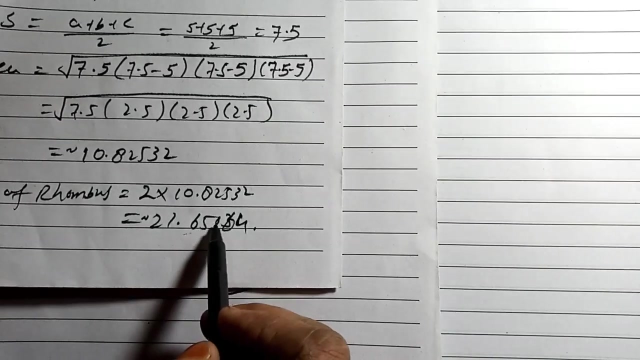 area of this robust and we left this for side so we can. so area of left side of triangle. so this is, if we see that at this side we can get on the poor side, which is equal to twenty one point six, six, five, zero, six, four. so the one side. 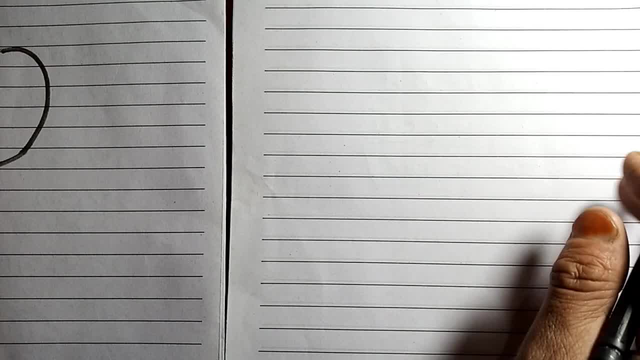 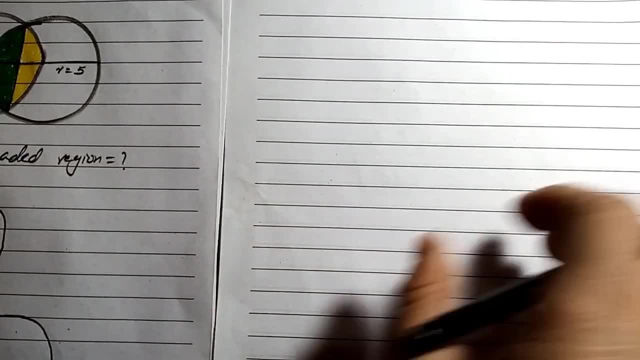 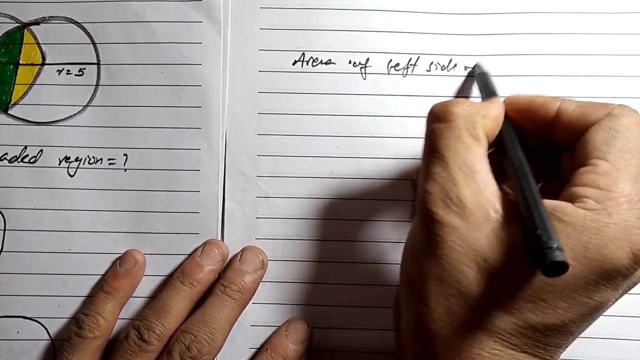 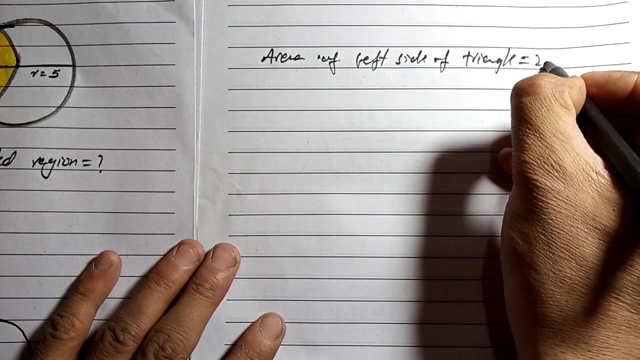 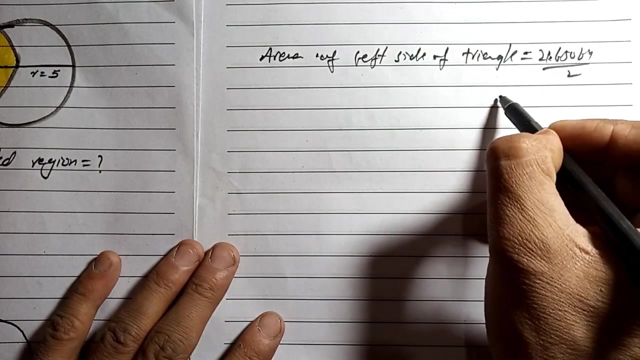 will be equal to, so we can find one side, so it half left side of triangle, area of left side of triangle, which is equal to twenty one point six, five, zero, six, four, divided by two, two time of the triangle, so you can get eight, five, three, two, which is one side. 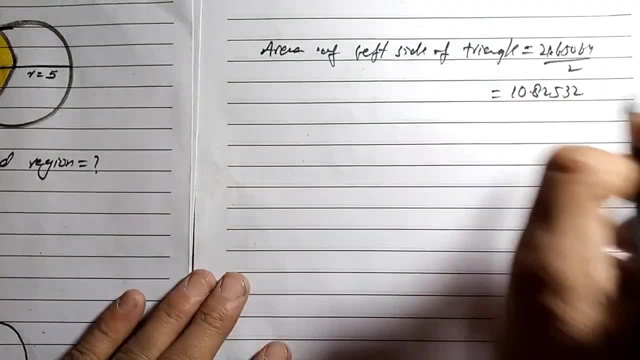 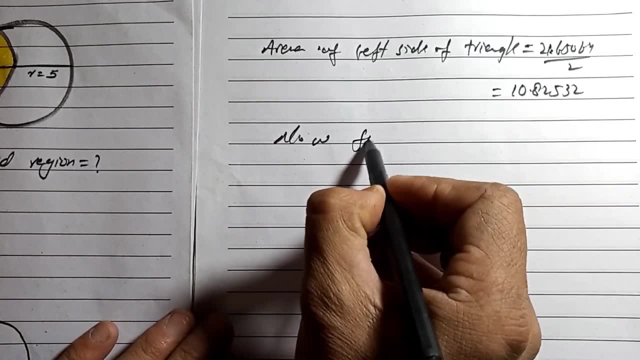 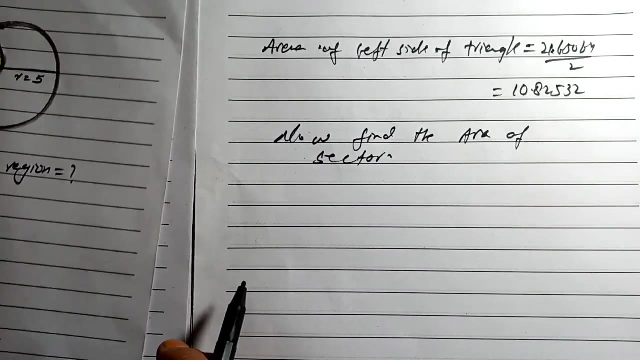 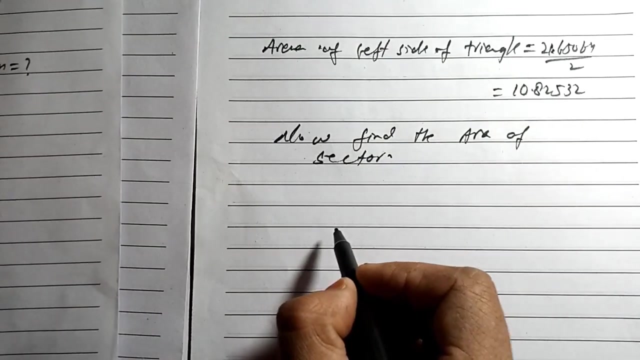 left side off triangle, so area. so now find the area of sector. no, we find area of sector, so we find here. it is not flexible. we thought this triangle would be OK. we found area of sector, so now we find area of sector, sector. if we see this shape, we can get: there is a sector, this is a sector, this. 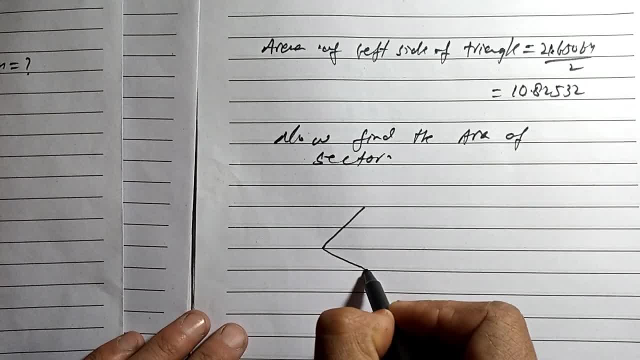 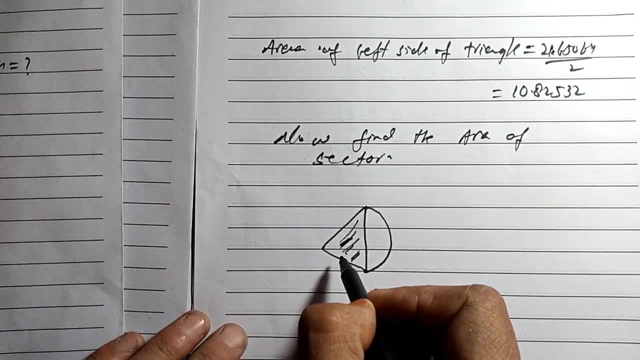 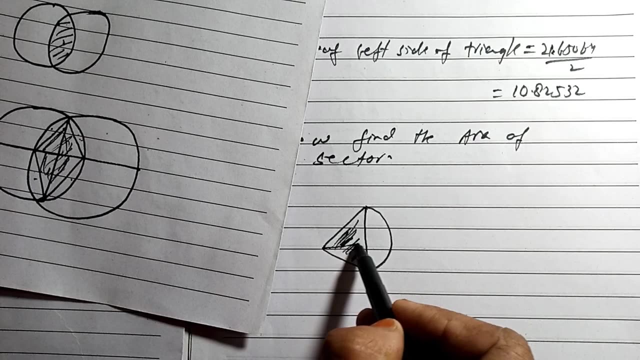 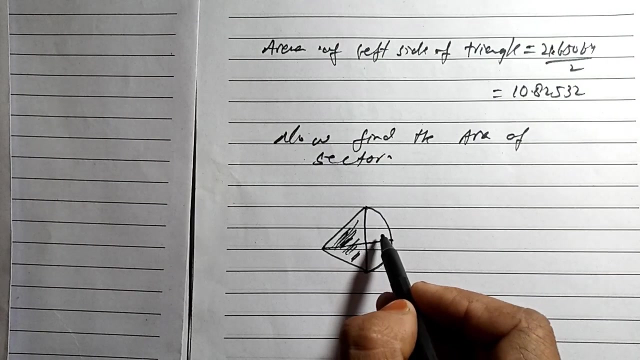 is shape of sector. this is a sector and we can get one side of, we can. we know that the one side, which is this two side, this is equal to this, is the only one side. this is a sector and this is a rhombus. so first we can find the area of 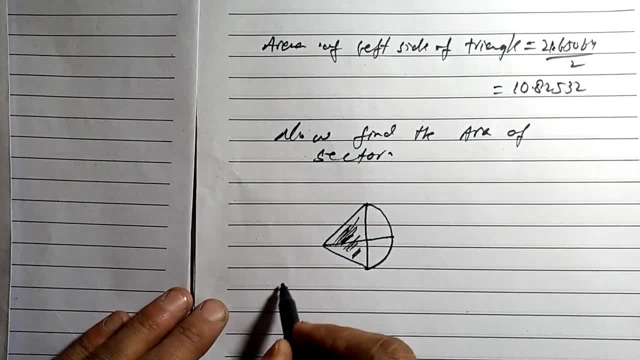 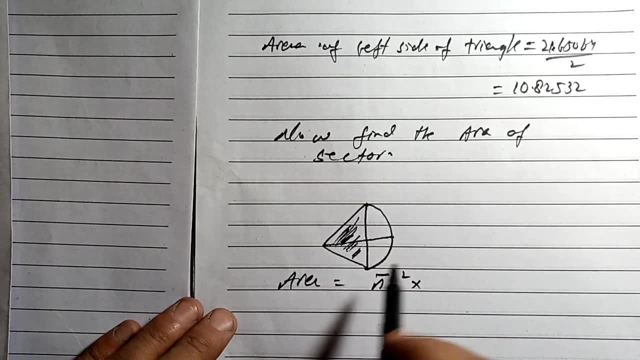 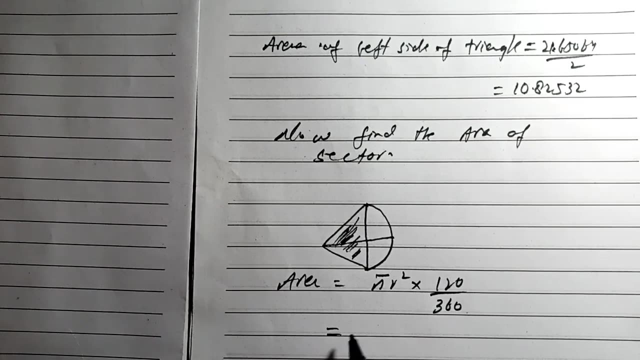 the sector, so area of sector. formula of area of sector, which is pi, R square multiply, there is 120 degree. total degree is 120, so 120 divided by 360. so then I get in the R which is 5, 5 square will play 120 divided by 360, so the total. 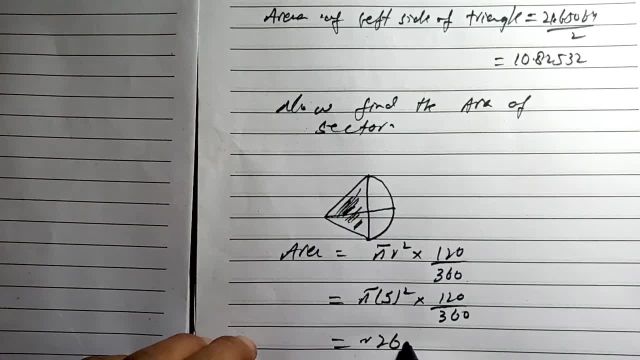 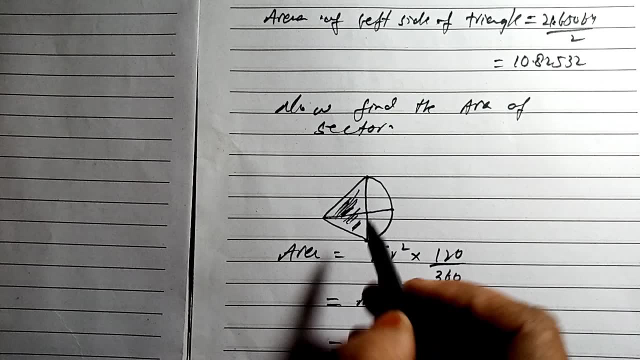 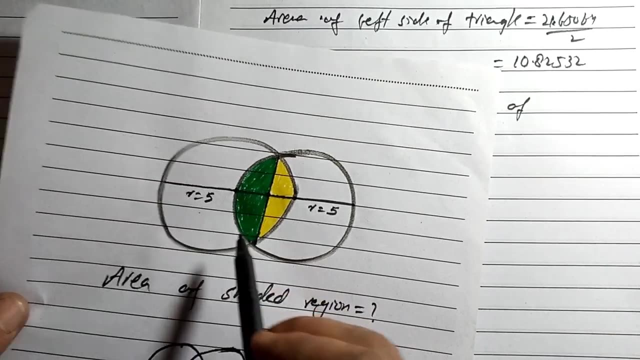 area will be equal to approximately twenty six point one, nine zero four it, which is the area of the total sector. so we can find the area of this site, we can find the area of this two side, these two side, which is equivalent. so this is one side. 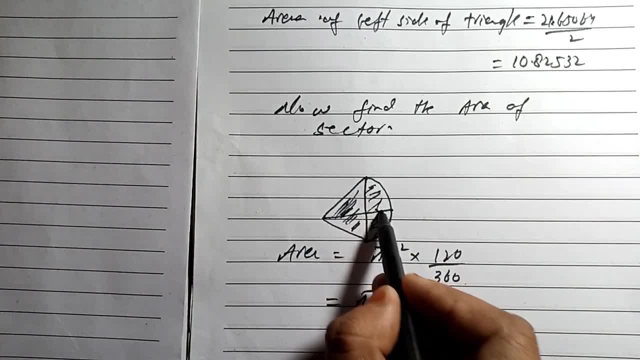 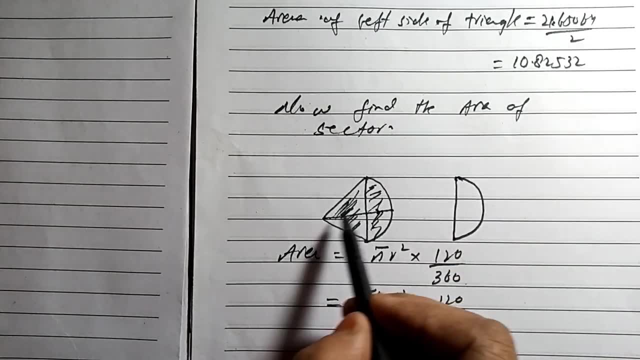 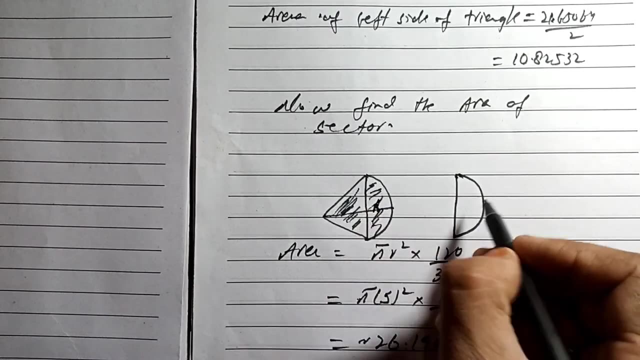 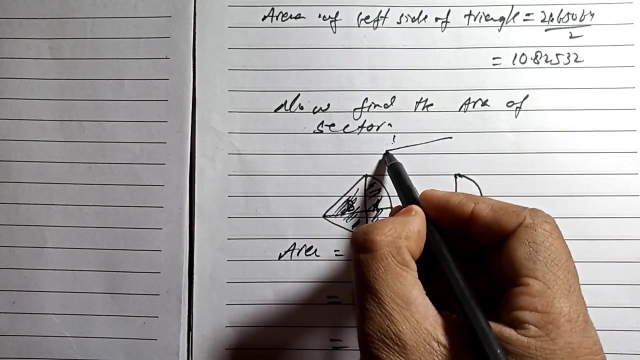 side side, so we find the area of this side, only this side, we can find the area of this side. so we know that the total area of this sector, which is equal to 26, so only this side we can find, we can name- this is a and this is b and the total is in the total sector we can name. 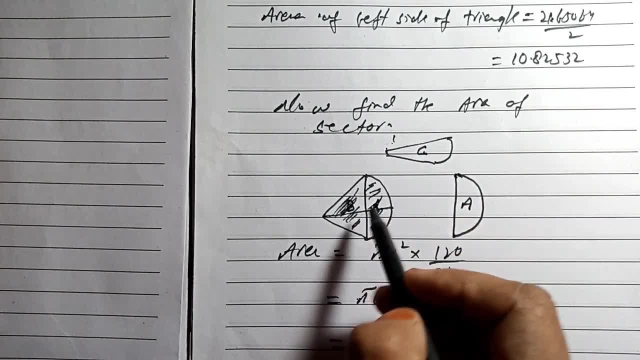 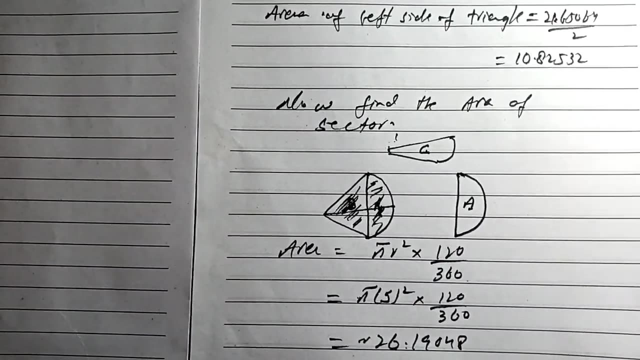 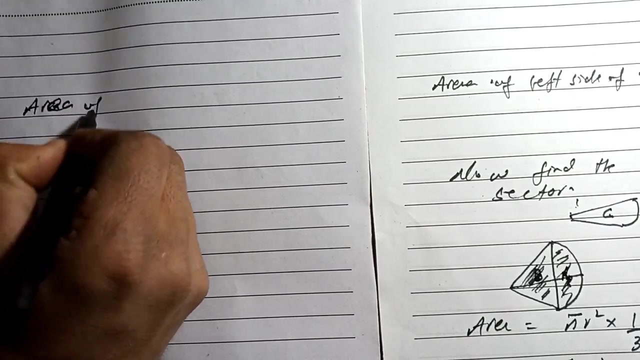 this is c, so total c. if we subtract c to p, we can get the area of this side, the total side. we can subtract this side, we can get this side, so we can find this a. so we can write here: area of a, which is equal to area of p. 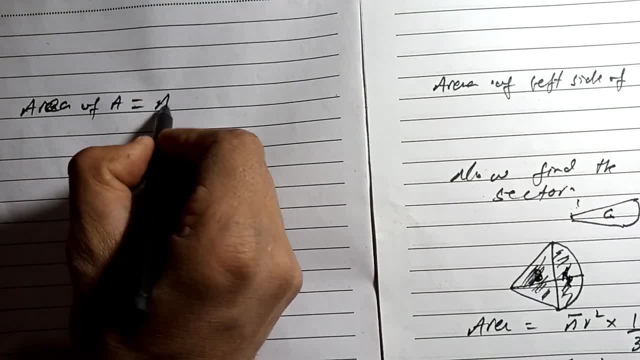 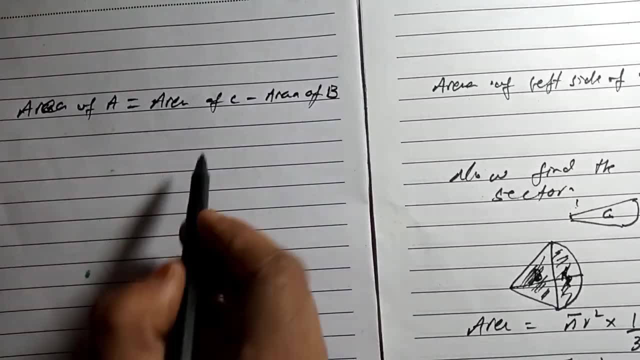 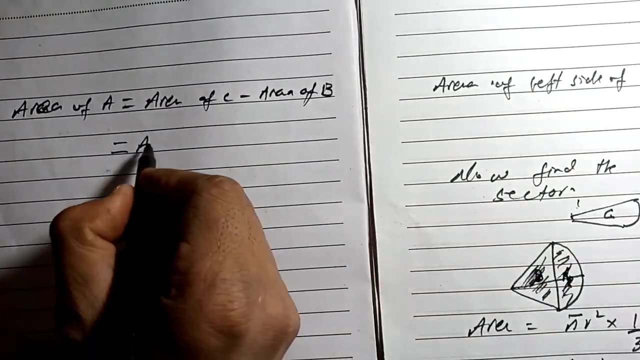 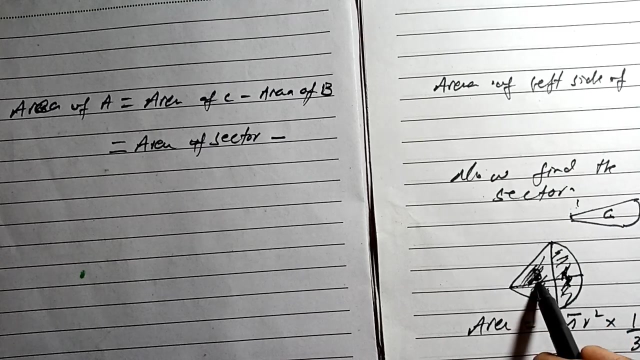 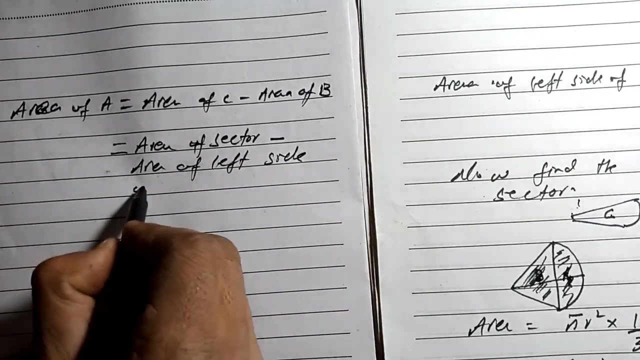 area of c. this is total area of c minus area of p. so area of c, which is total sector c, which is equal to total sector, area of sector sector, minus area of b, which is the left side of triangle, left side of triangle, area of left side of. 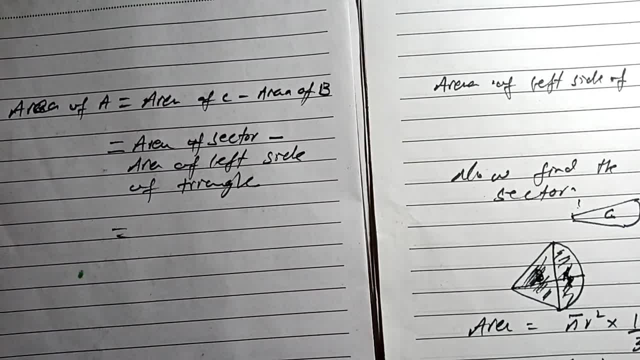 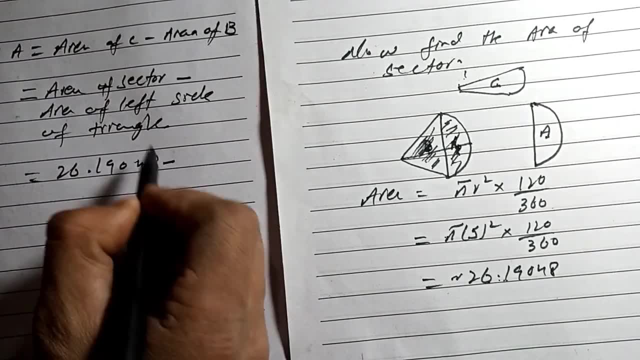 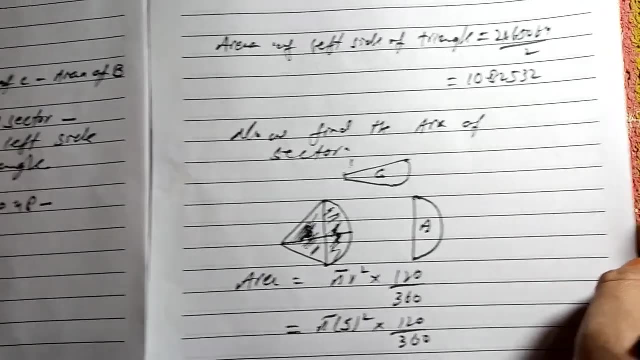 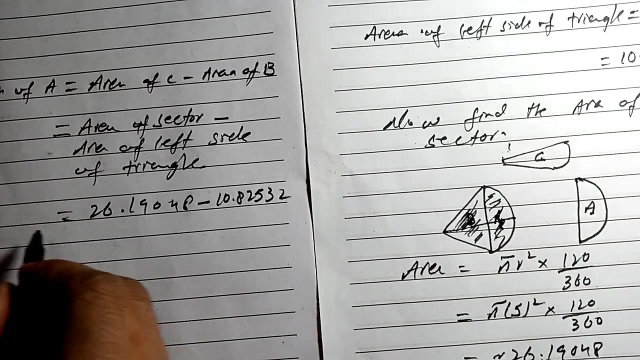 triangle. so area of sector we can get here, which is 26.19048, minus area of left side of triangle. we can find here 10.825, 10.82532, 82532, so we can get the area of this side, the, a area of a.